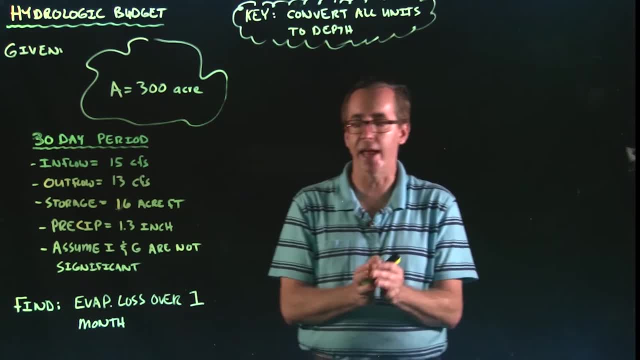 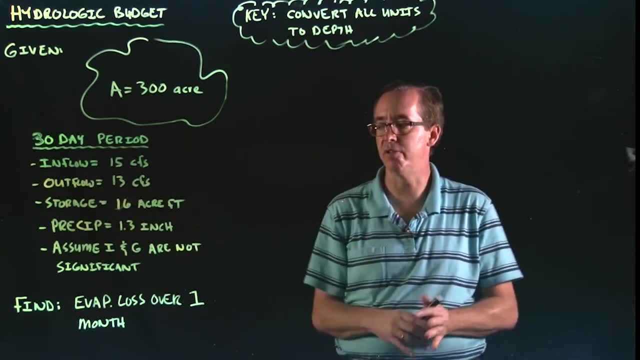 Of course there are some values, but we're just assuming that numerically, their values are very small relative to the inflows, the outflows, the storage and the precipitation. And what we want to know is: over that one-month period, what did we have in terms of evaporation? 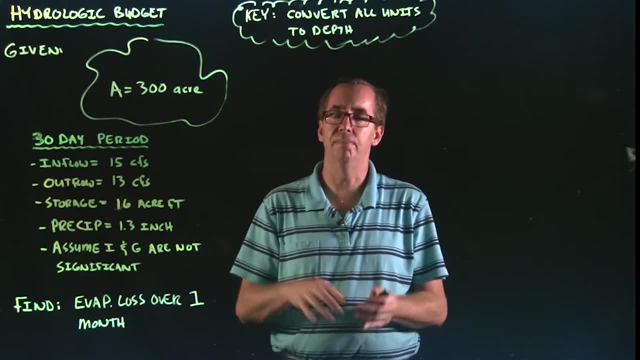 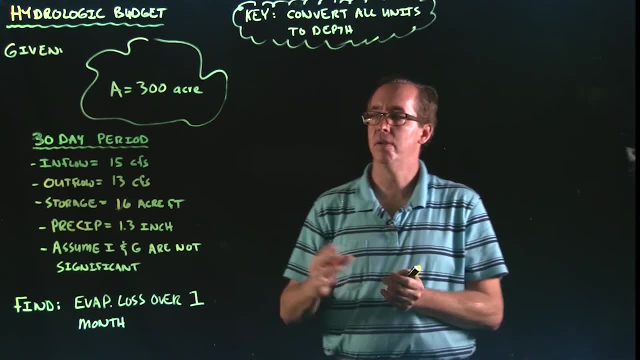 Now, the key to any of the hydrologic problems- of course, the budget problems- is converting all these different units into the same set of units, And what we usually do is we convert everything to depth. So, for example, these flows in CFS we'll convert to depth. 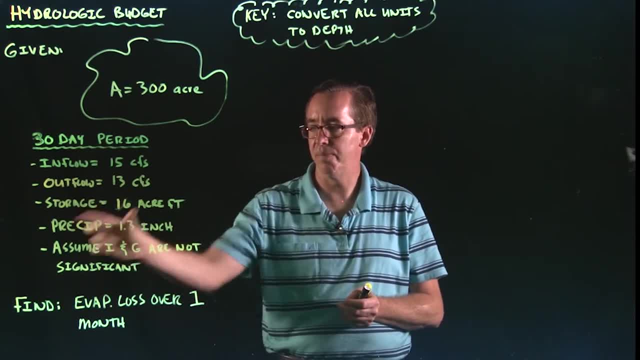 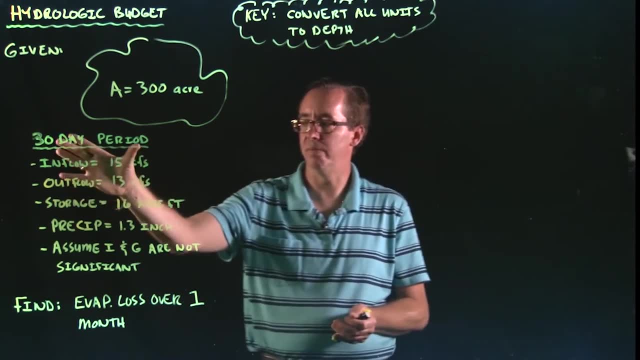 The storage in acre feet, we'll convert to depth and so forth. Precipitation already is in depth, But that will be the process. So I'm just going to start by item by item, going through and converting all these units into the right units. 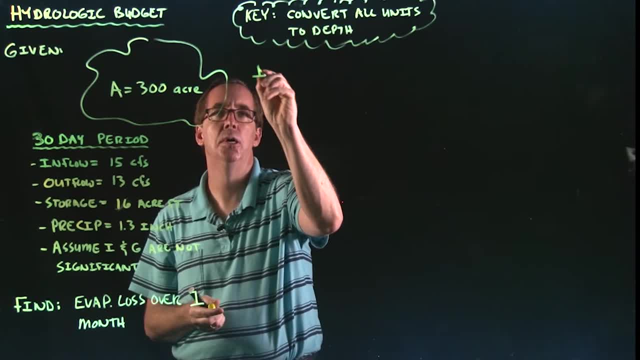 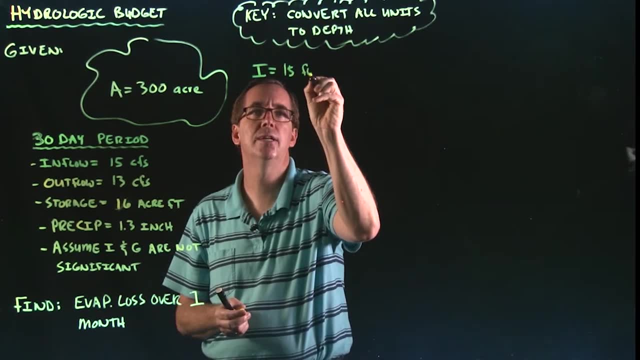 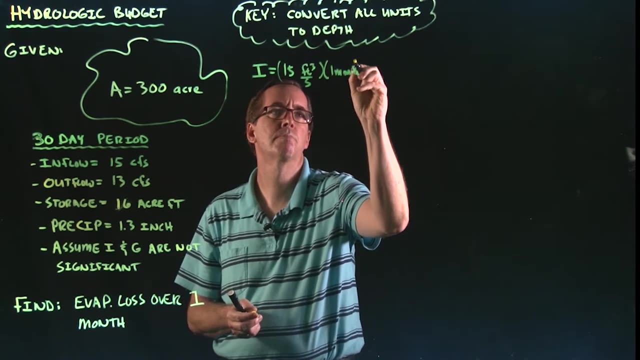 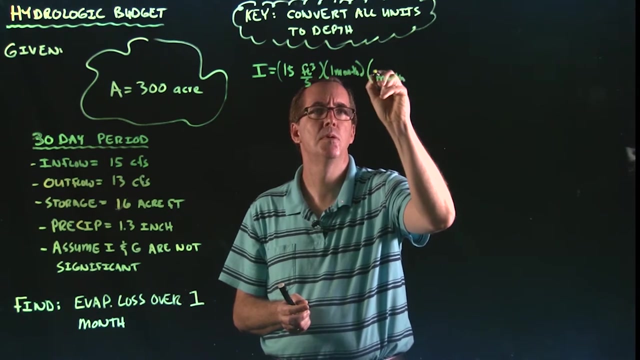 So for inflow, I've got, let's see, 15 cubic feet per second. Okay, Over a one-month period, Okay. And then we just start going through and saying, okay, in a month. Let me switch markers here. 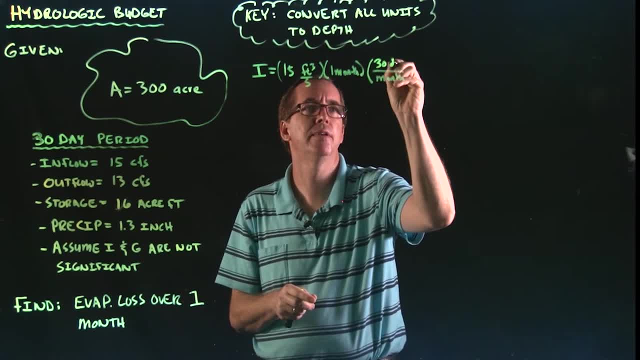 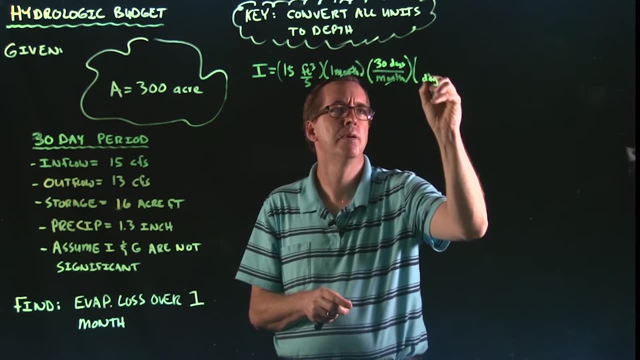 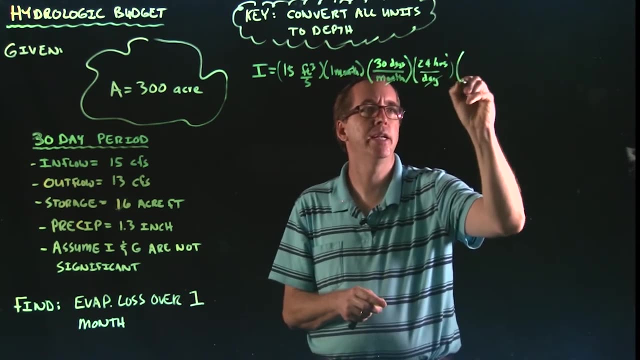 That one's a little squeaky. We have 30 days- Okay, So the amounts cancel In a day. we've got 24 hours- Okay, So my days cancel In an hour. we have 3,600 seconds. 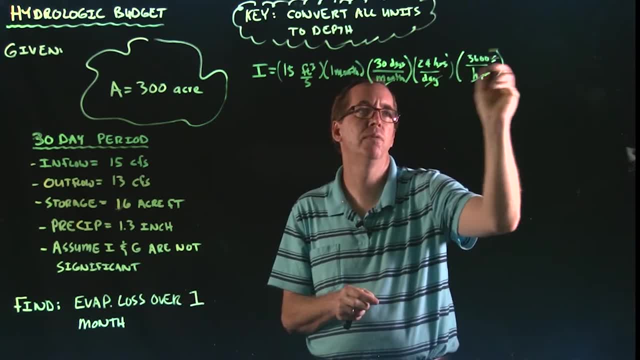 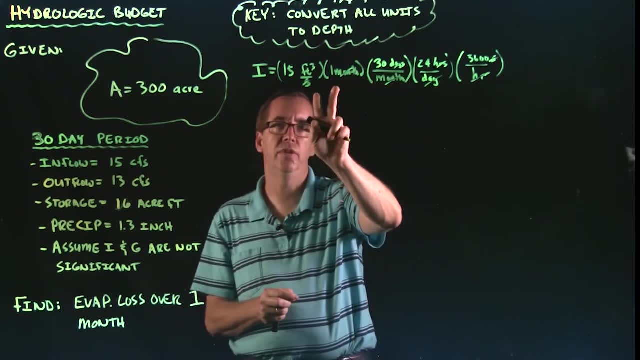 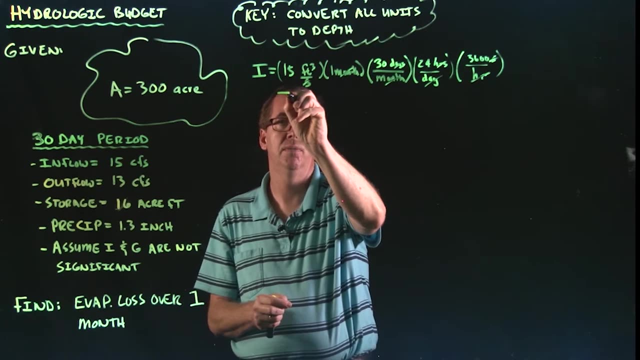 So my hours, let's see right, here's hours and we've got seconds and seconds. Okay, So let me make sure we've got the infiltration That gives me the inflow of this And we're going to take this and we're going to divide it by 300.. 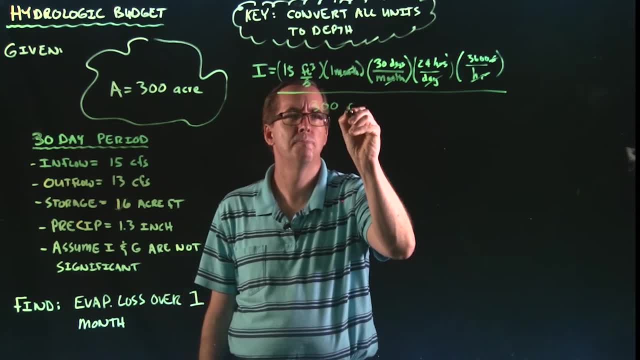 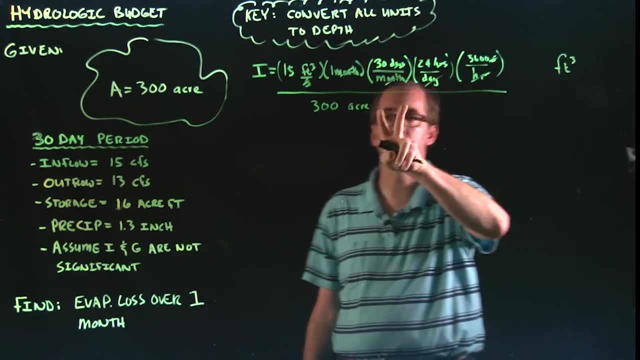 So we've got 300 acres, Okay, So right now, the numerator. I have everything in terms of cubic feet, So what I want to do is get the denominator by square feet and then I can divide that out. I'll have a depth in feet and we can convert that to inches. 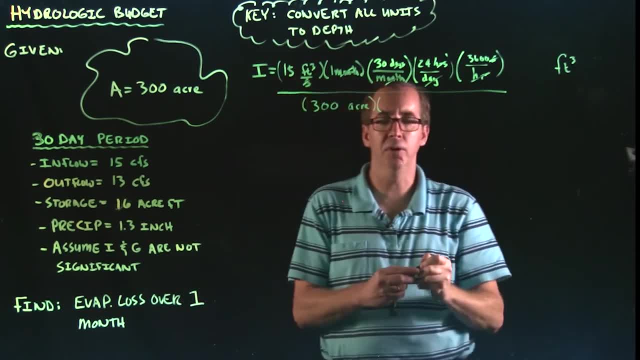 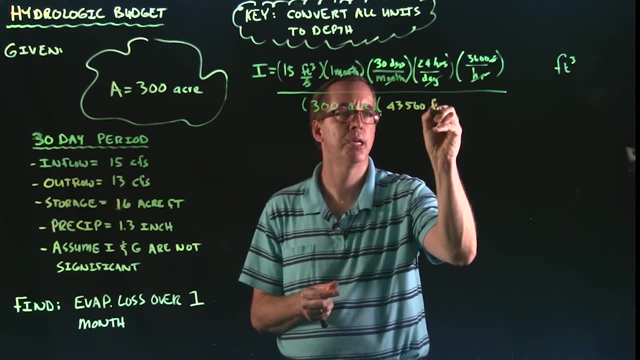 So we have 30 acres. One of the main conversions that we use in this classroom- we use this all the time- is that in an acre we have 43,560 square feet, So we're going to convert that to an acre. 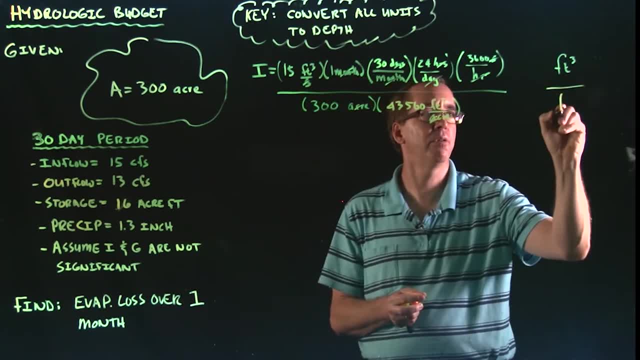 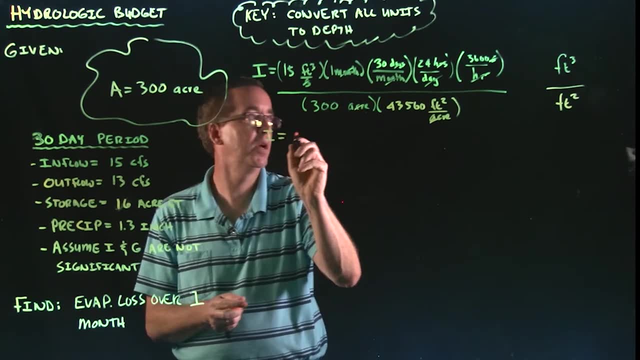 Okay. So again, when I do this, that leaves me the denominator of square feet. I have cubic feet in the numerator And what that does is that gives me a final value of my inflow. It comes out to be 2.975 feet. 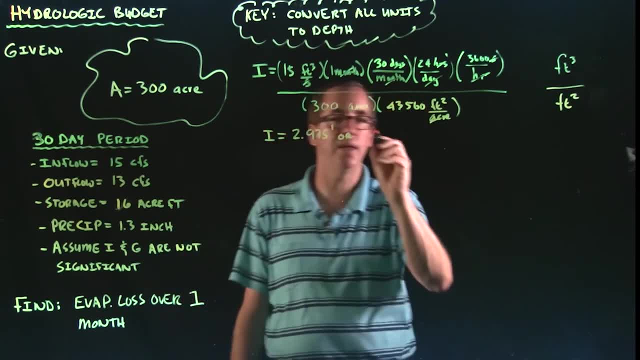 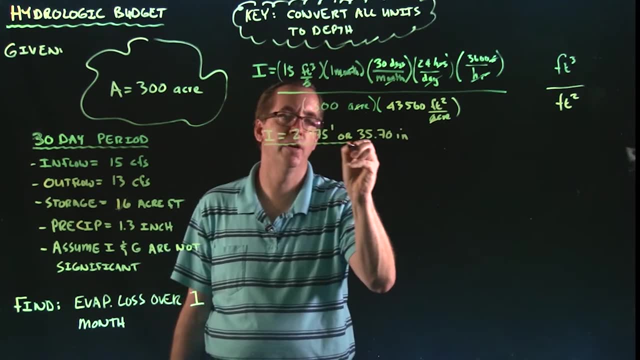 Okay. Or in inches, that comes out to be 35.70 inches, Okay, So. So I'm going to divide everything into depth. for the inflow, So that's this value here. I'm going to do the same thing for the outflow. 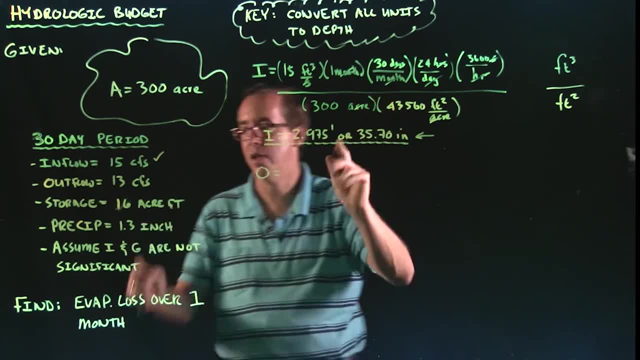 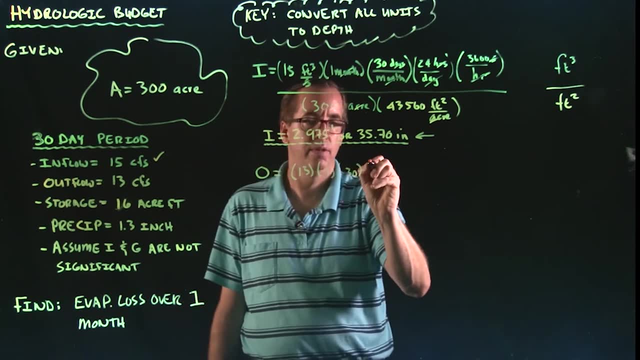 Of course, in this case I'm not going to worry so much about writing all the units out, I'm just going to do the same conversion. So you have 13 times 1 times 30 times 24 times 3,600.. Again, everything else is the same, And you divide that by the 300 and then the 43.50.. I'm sorry, 43,560.. And we get for depth, we get 2.578 feet, which in inches is 30.94 inches. 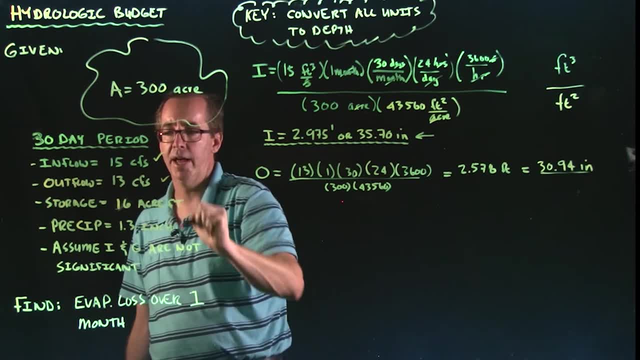 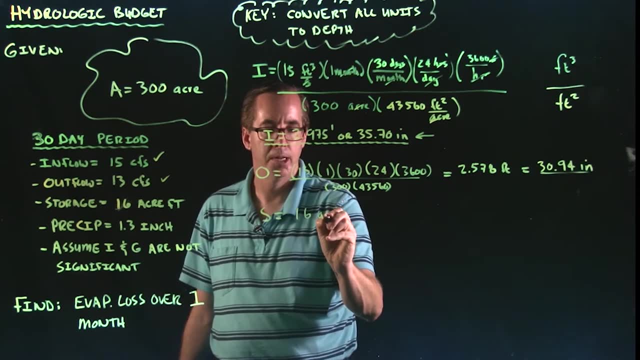 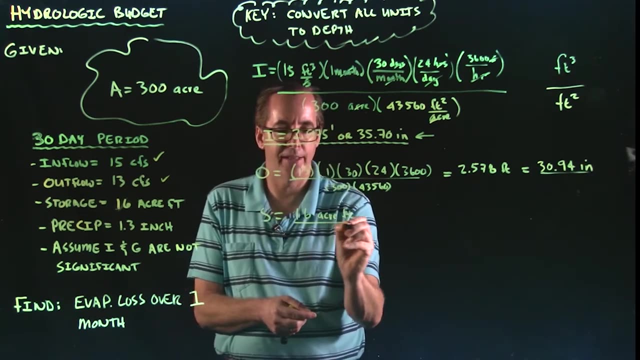 Okay, So here we've got that. One more thing for the storage: Okay, We have 1,600 acre feet. Okay, That's a volume, right? So we're going to take that, We're going to divide that by the number of acres that we have, which is 300 acres. 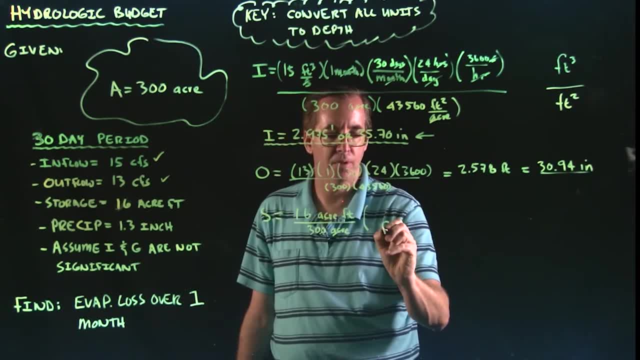 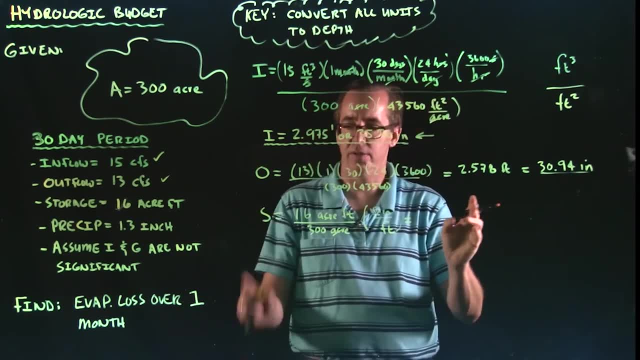 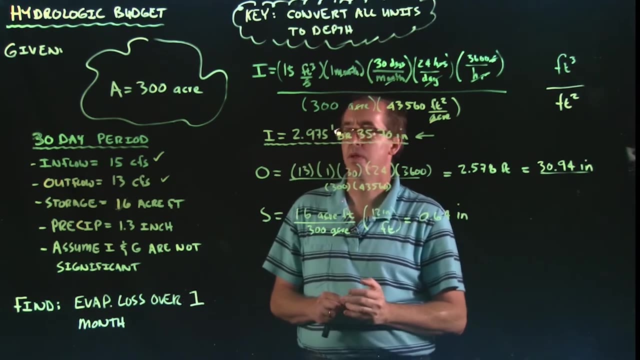 Okay, That will give us feet, And then we'll convert feet into inches. Okay, And that gives me a storage comes out to be 0.64 inches. Okay, So we've got all this in inches And we're ready to rock and roll. 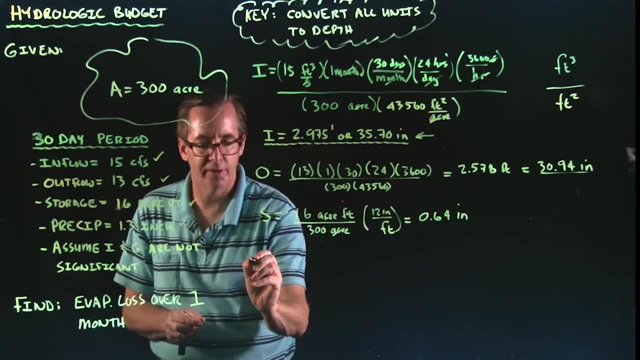 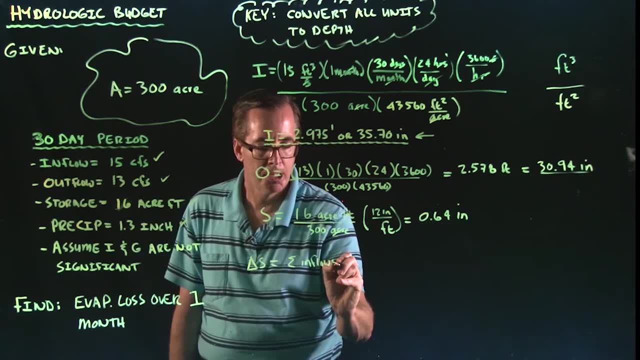 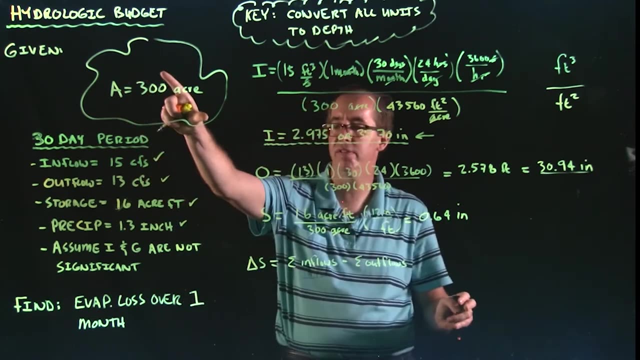 So for us to do our balance, the main equation is that the change in storage is the sum of all the inflows minus the sum of all the outflows. Right, So we're just saying whatever storage change we have for this lake is just the sum of everything. 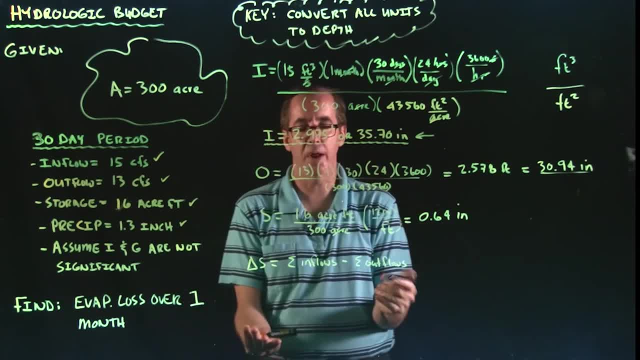 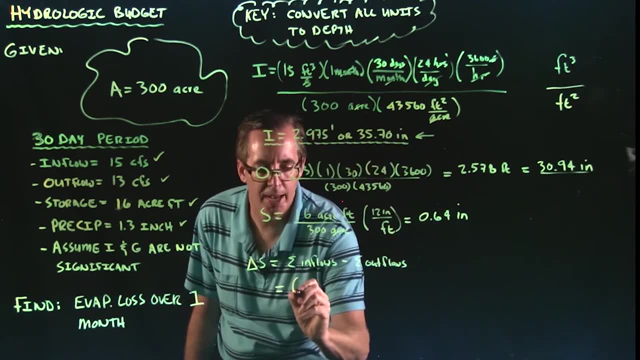 that's flowing into the lake, minus everything that's flowing away from it. Okay, So for the inflows, of course our first inflow is going to be 0.64.. Okay, So for the inflows, of course, our first inflow that we have is we have the 35.70 inches. 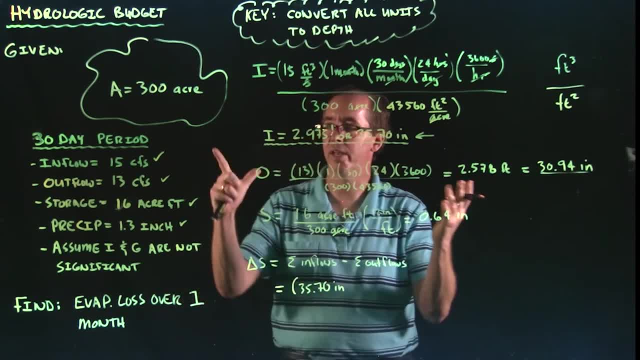 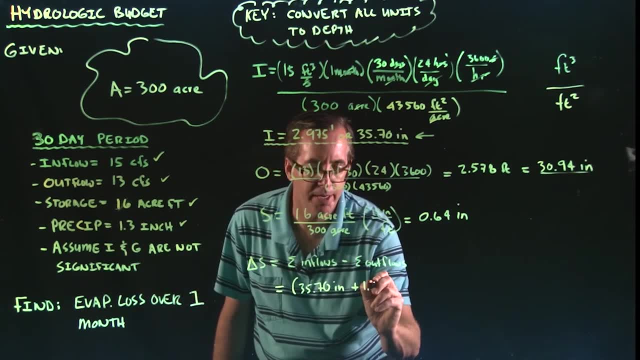 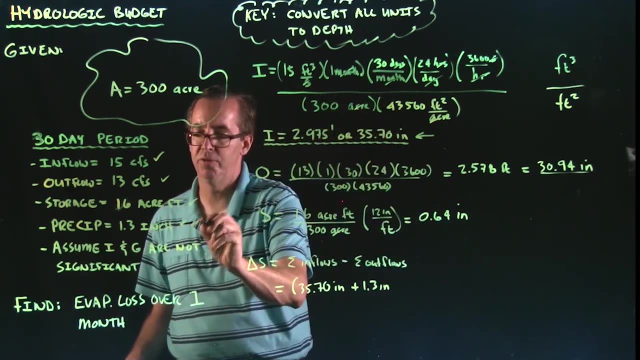 Okay, That's an inflow. What else is flowing into it? That would be precipitation. Okay, Precipitation in this case is 1.3 inches. Okay, Those are the only things we have, So I'm just going to do a double check here to make sure I'm getting all these values. 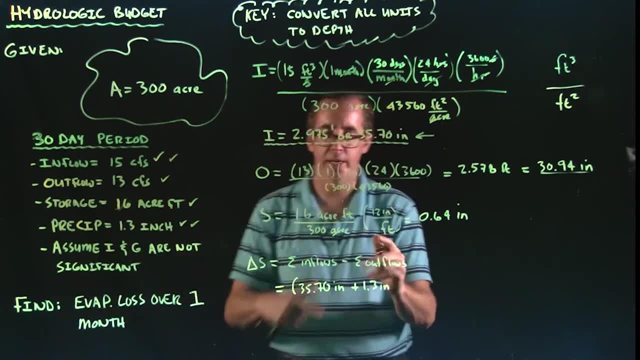 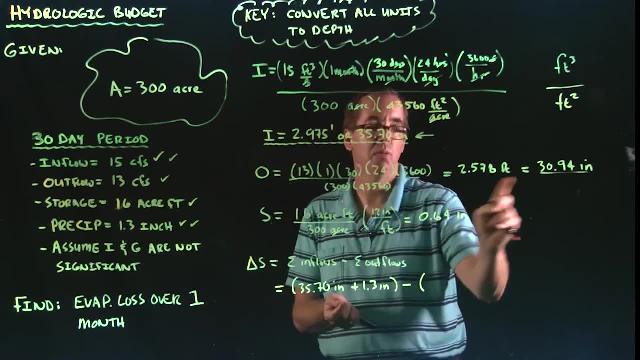 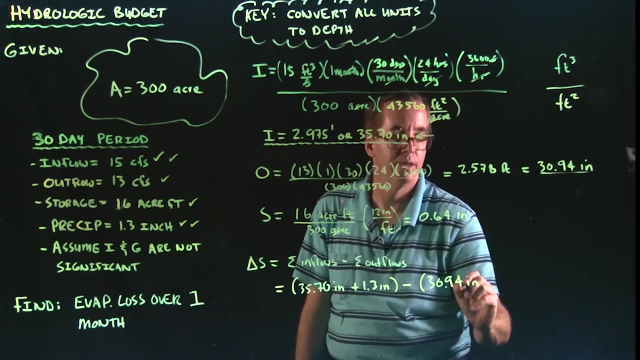 Okay, So that's what's flowing in- Okay, Minus. and then we're going to talk about what's flowing out. Okay, We have an outflow here of 30.94 inches. Okay, That's our outflow. 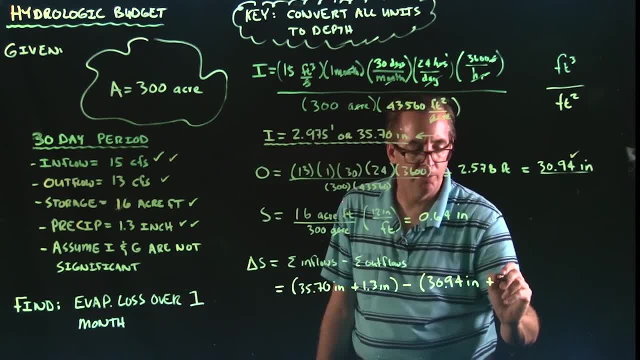 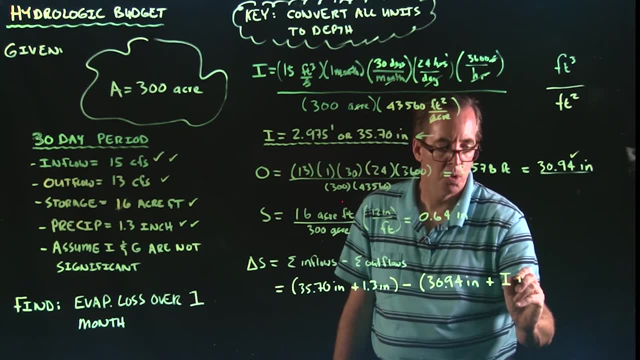 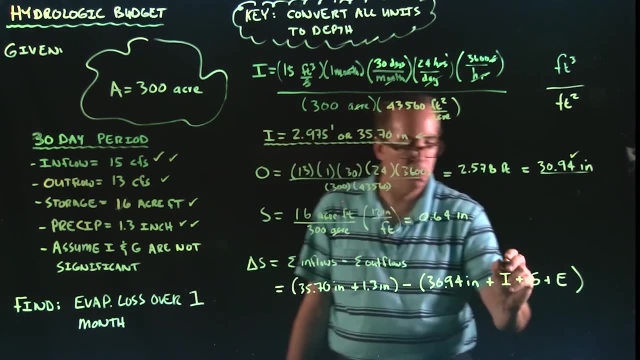 Now normally again, we would say: well, you know, we've got the inflow of flow going into the soil beneath it, right, the inflow. We have groundwater flow and we have evaporation And, as I mentioned earlier, we're going to assume that the inflow and the groundwater 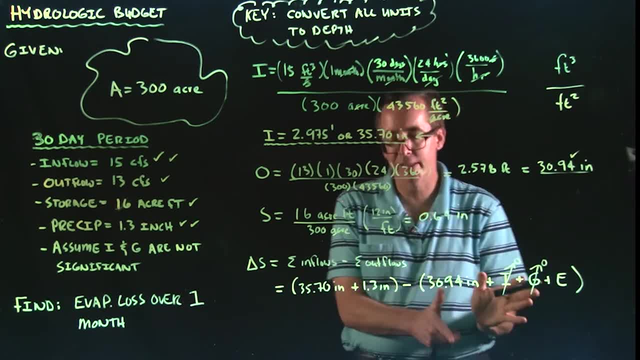 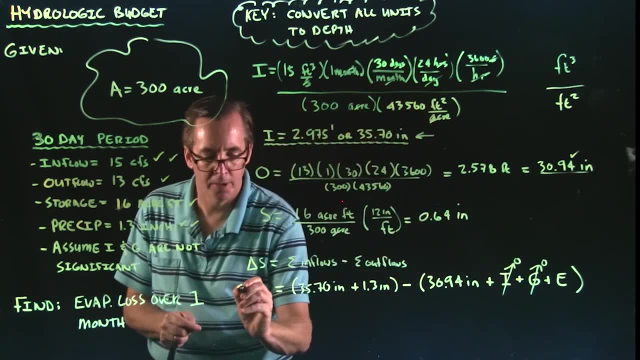 flow are 0.. No, they're technically not 0, but they're very small relative to all these other values. Okay, And we know our storage is 0.64 inches. Okay, So all we have to do now is basically just solve that. 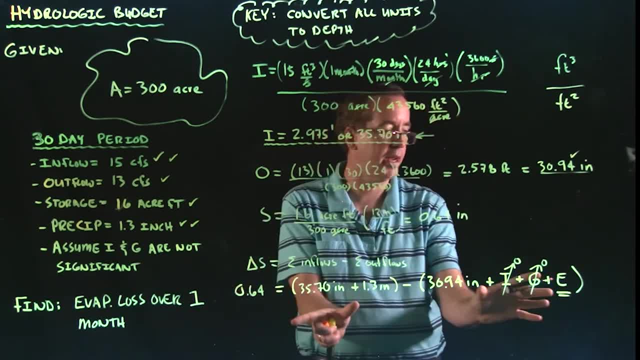 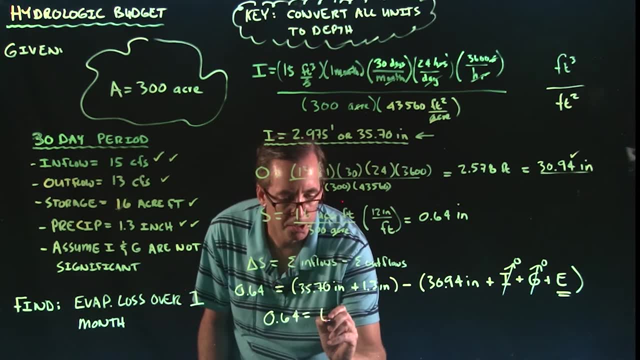 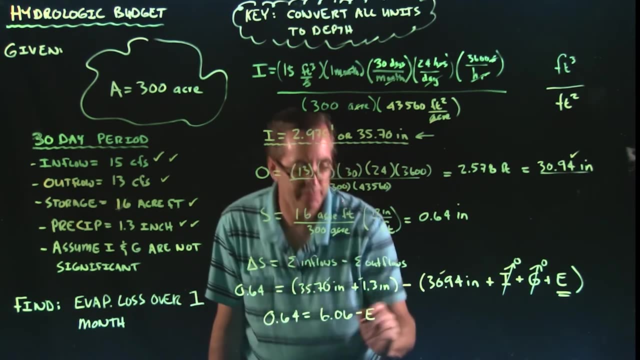 Right, Knowing the left-hand side, just solve it with the right-hand side. I get one more thing. I get: 0.64 is equal to 6.06.. Right, All these minus that comes out to 6.06. minus the evaporation, or evaporation comes out. 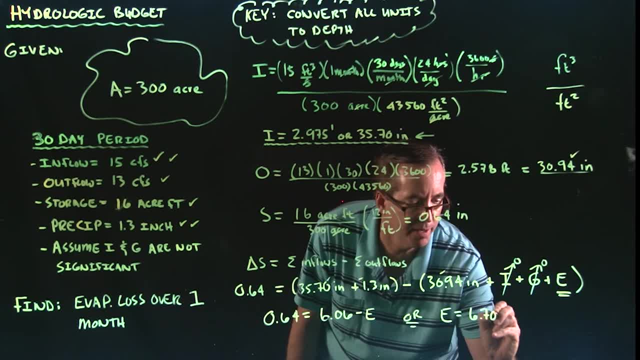 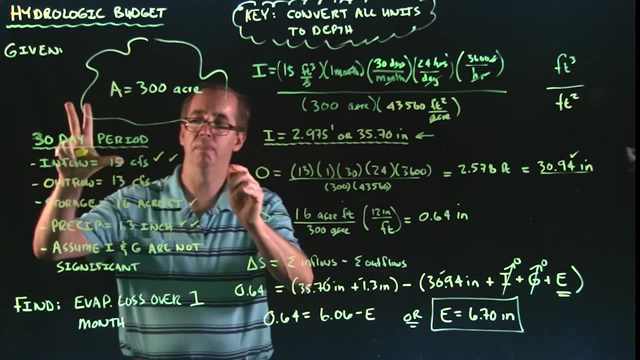 to a final value of 6.7 inches. Okay, So again, to reiterate, what we did is: we looked at this problem. We looked at all the inflows and the outflows. The key was converting everything into the same units because we had cubic feet per. 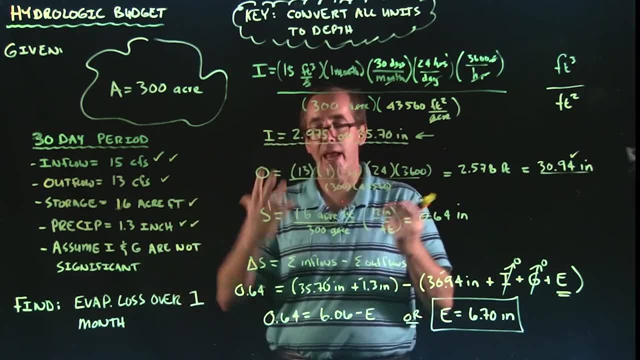 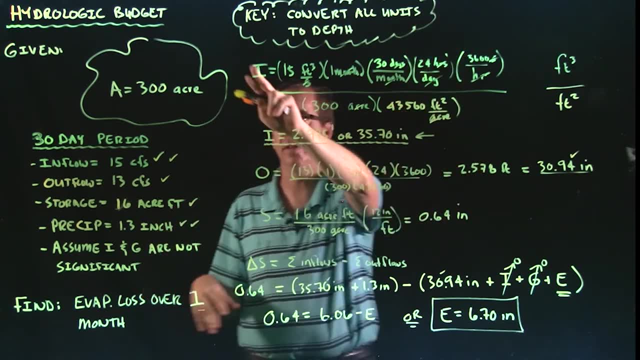 second, We had acre feet, We have inches And we just we can't add apples to oranges, So we have to convert everything into the same units, which we did of units of depth. In this case it was inches, So I converted the inflow, the outflow, into inches.